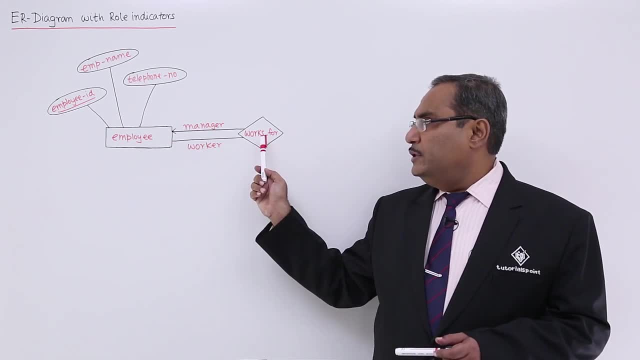 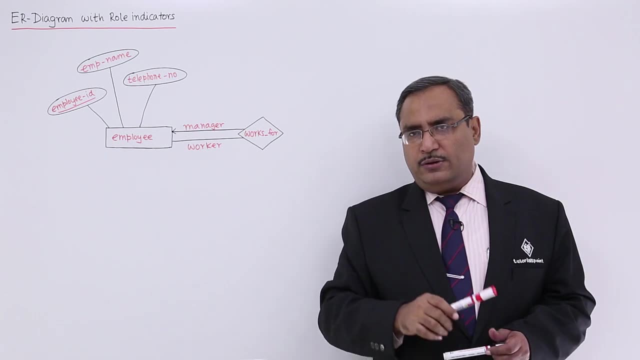 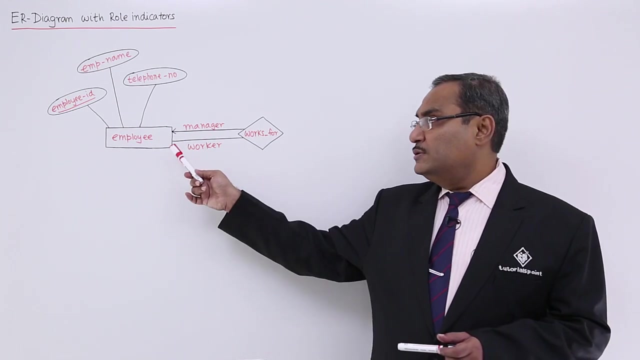 that one entity has got connected with this relationship twice. So when we discuss our relationship and relationship sets in that particular video, we told you that entities connected with the relationship may not be distinct. And here you see, this entity is not distinct. The same entity has got connected with the relationship more than once. 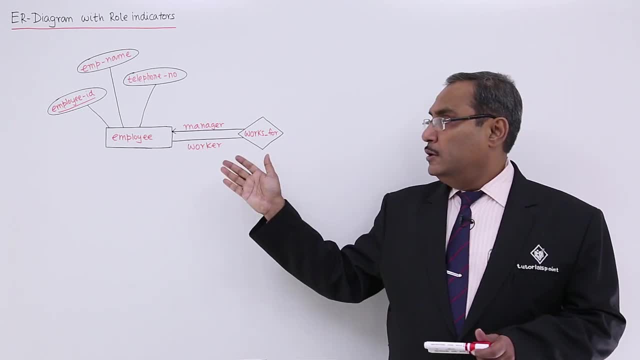 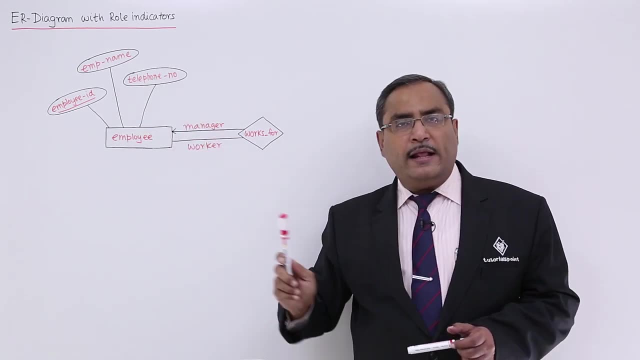 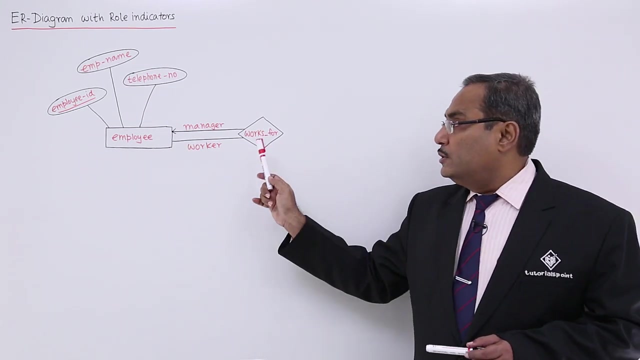 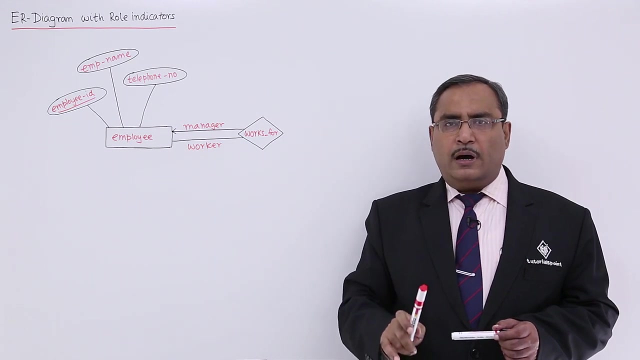 Now, what is the issue? What is the logic working behind this? Employee is one entity having got three attributes: employee id, employee name and the telephone number. Good, So Here, employee ID is the respective primary key. So now see, irrespective of the fact whether the person is manager or worker, all of them. 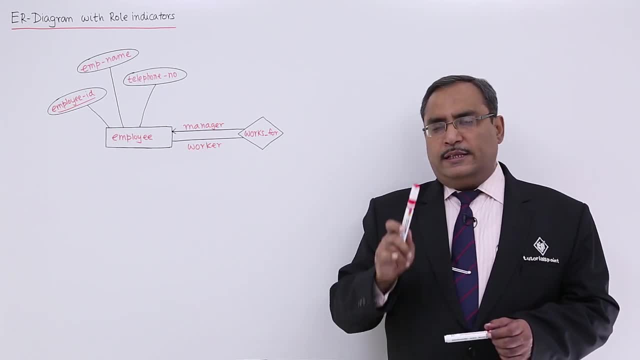 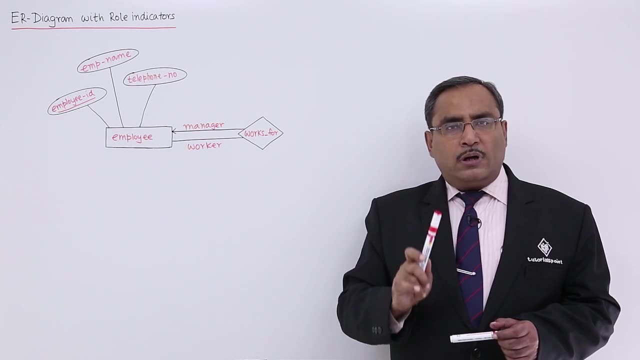 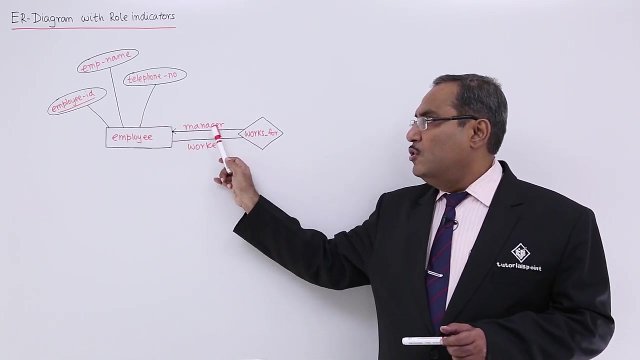 are the employees of the company And we know that these manager details and worker details will be there only in the employee table. Under one manager, multiple workers are working, So manager is one and workers are many, So that's why this arrow is being directed from worker to manager. 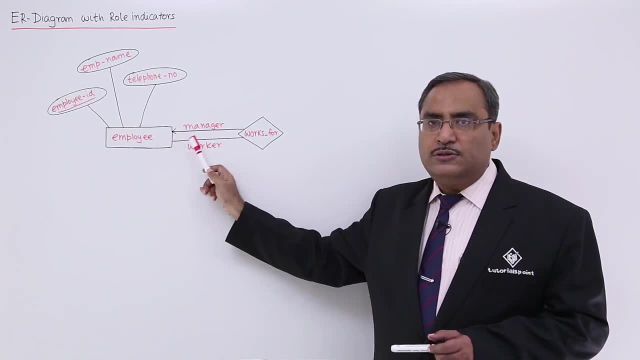 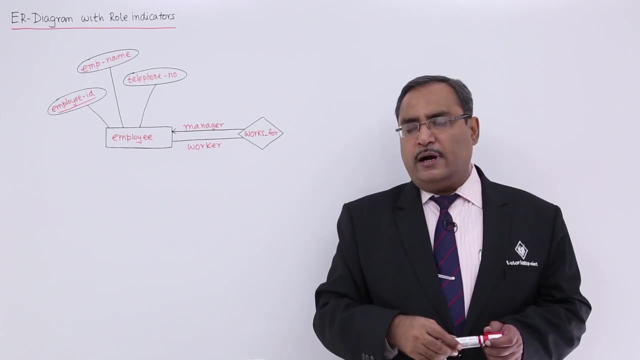 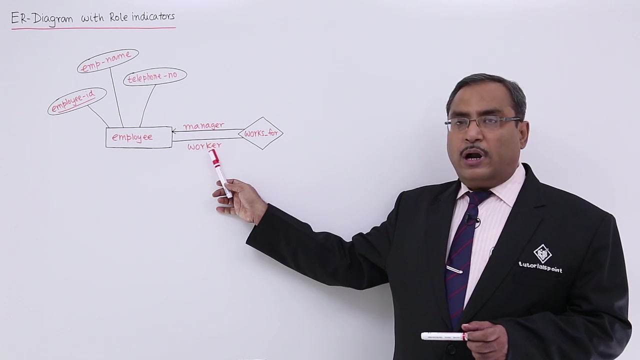 As manager is one, so array will be there. As worker is many, so there will be no arrow. Just watch the previous video where we have discussed this mapping cardinality, how the mapping cardinality can be expressed in our year diagrams. Okay, now the thing is that, as worker is many and manager is one, so against one manager. 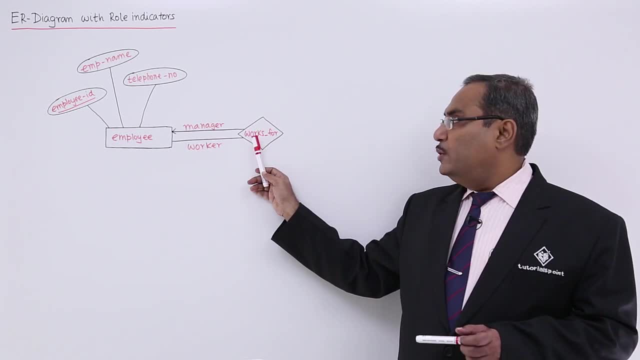 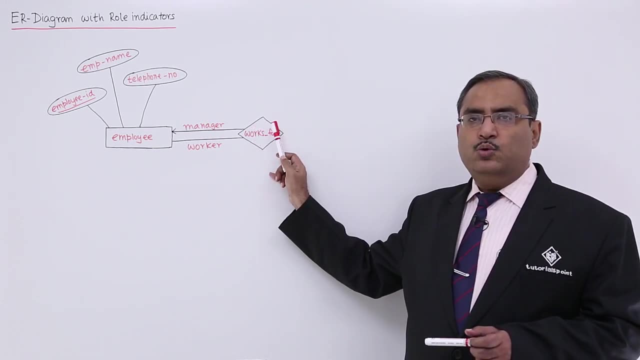 ID. we are having multiple worker ID. So in this particular relationship set we are having like this one. say, E1 is one of the manager's ID, E2 is one of the worker's ID. So it will be written in this way: E1, E2, E1, E3, E1, E4, E1, E5, because E1 is the manager. 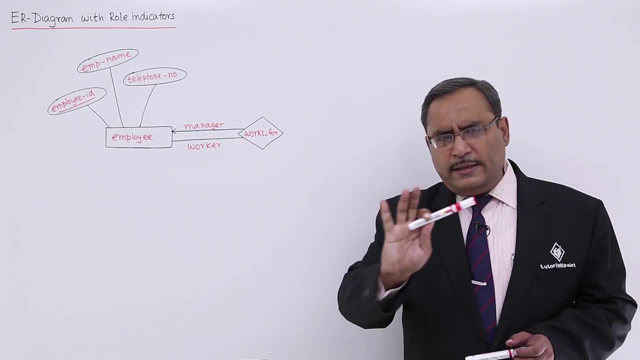 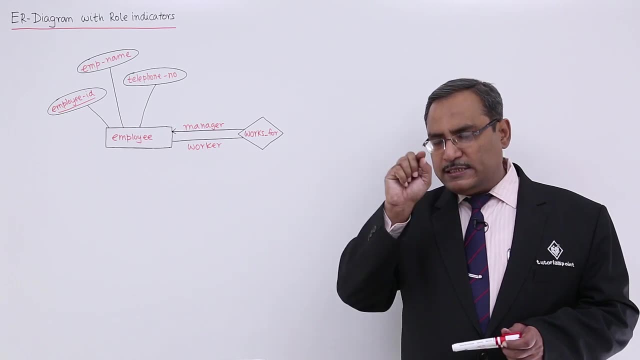 ID and E2,, E3,, E4, E5, let there be the worker IDs. So that's why we are having this E1 for multiple number of times occurring against multiple worker IDs. So that sort of relationships will be formed and collection of them will be getting this.